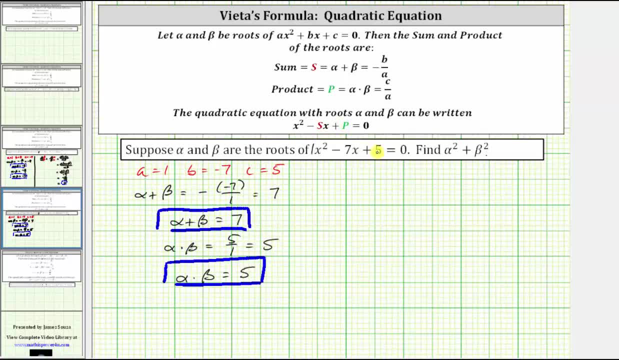 by using the constant term. and notice how here the constant term is five, which does give us the product, But this does only work when the leading coefficient is one. And now let's determine the value of alpha squared plus beta squared. Notice how we cannot evaluate the expression in this form. 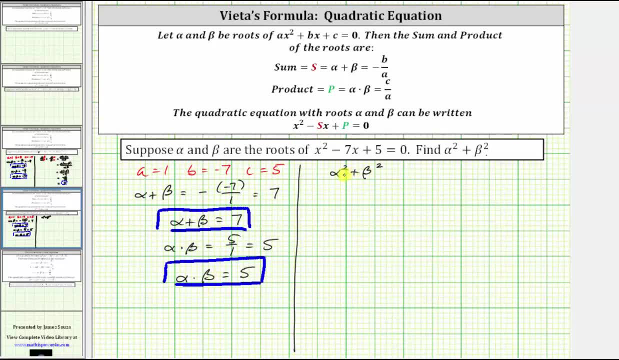 because we don't have alpha squared. We only have alpha squared or beta squared, So this one's a little bit tricky. We're actually going to consider the square of alpha plus beta. Well, the square of alpha plus beta is equal to two factors. 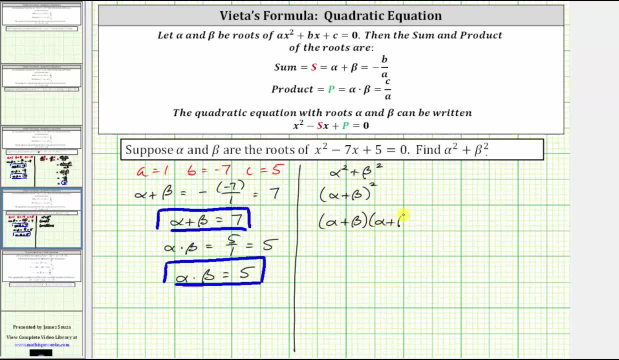 of alpha plus beta Again. this might not make a lot of sense now, but it will in a moment. And now we multiply. We have four products: one, two, three and four. This is equal to alpha times alpha. 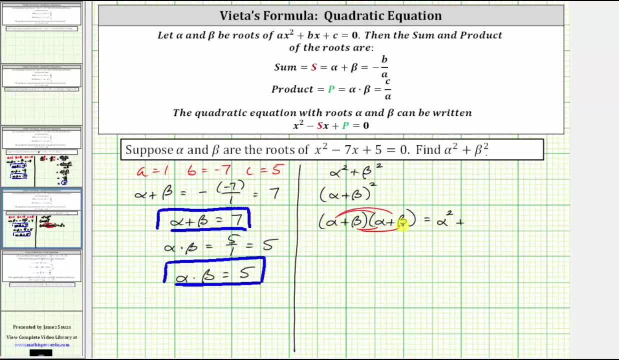 plus alpha squared, plus alpha times beta, which is alpha beta, plus beta times alpha, which is another alpha beta. So we have plus two alpha beta and then we have plus beta times beta, which is plus beta squared. Notice, on the right side of this equation. 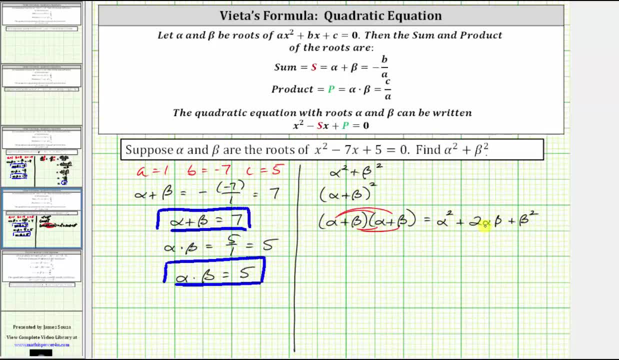 we do have an alpha squared plus beta squared, but we also have this plus two alpha beta. Let's subtract this on both sides of the equation. If we subtract two alpha beta on both sides of the equation, we have two alpha beta on both sides. 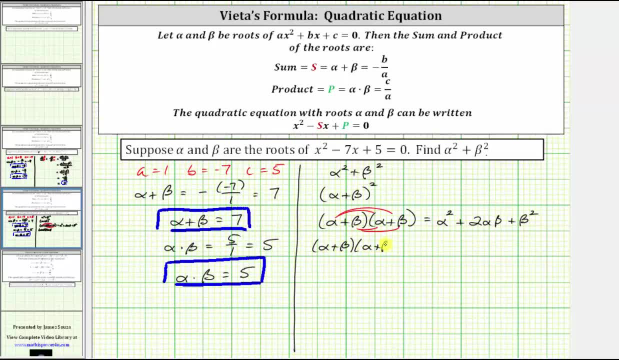 We have alpha plus beta times, alpha plus beta minus two. alpha beta is equal to alpha squared plus beta squared. And now we can determine the value of alpha squared plus beta squared by using the expression on the left. We know alpha plus beta is equal to seven. 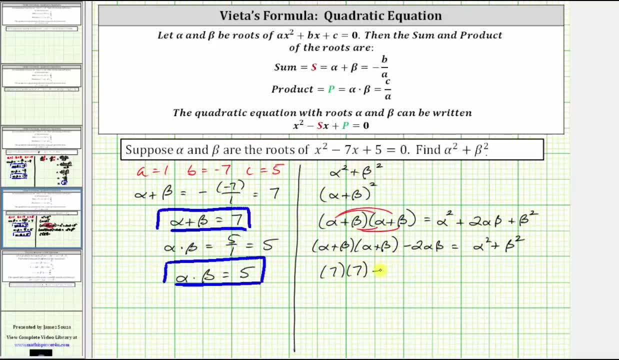 So here we have seven times seven and then minus two times alpha times beta. alpha times beta. Two times beta is equal to five. So we have times five and this is equal to alpha squared plus beta squared. Well, seven times seven is 49,. 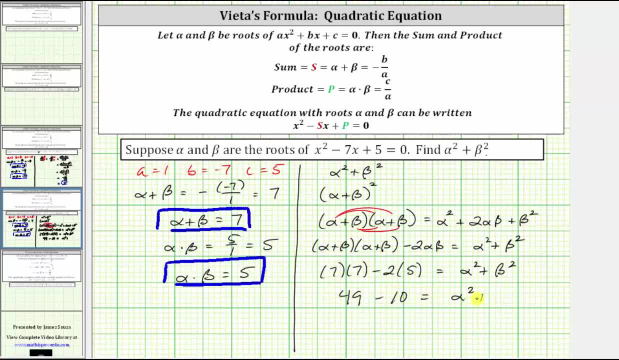 and two times five is 10.. So now we know that alpha squared plus beta squared is equal to 39.. I hope you found this helpful. If you did, please like, comment and subscribe And I'll see you in the next video. Bye-bye.